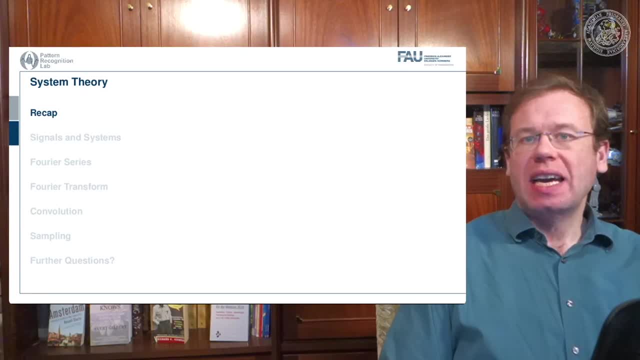 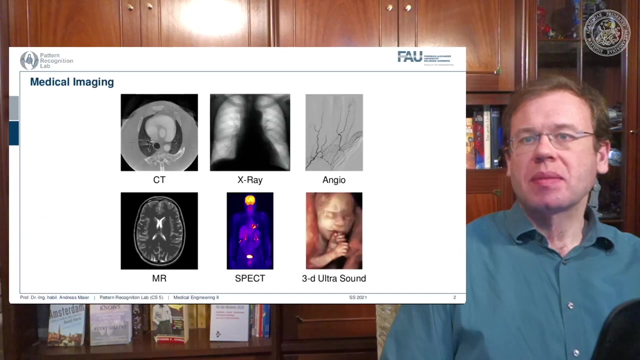 why we actually need systems theory and what kind of images we're dealing with, what kind of data we're dealing, what we're dealing with in medical imaging and why systems theory might be useful to understand the general basics of our systems. So you remember that we had the different imaging modalities and 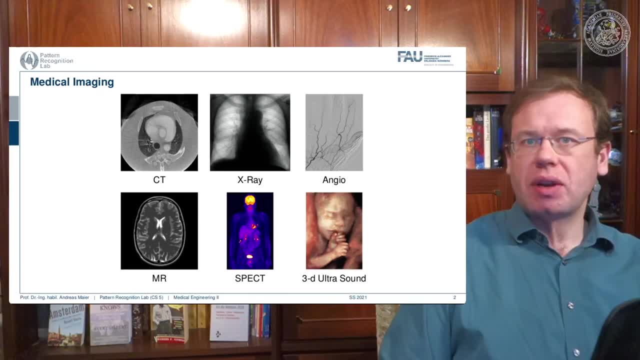 those modalities had very different appearance, they had very different contrasts and we've seen the examples from CT to x-ray, to angiography, MR, SPECT and also ultrasound. So we've seen we have many different imaging modalities and we've seen a lot of different imaging modalities and we've 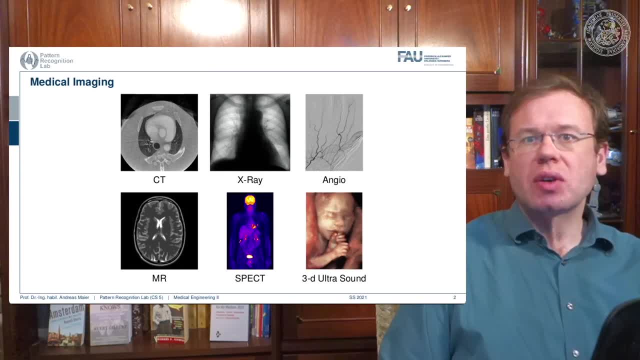 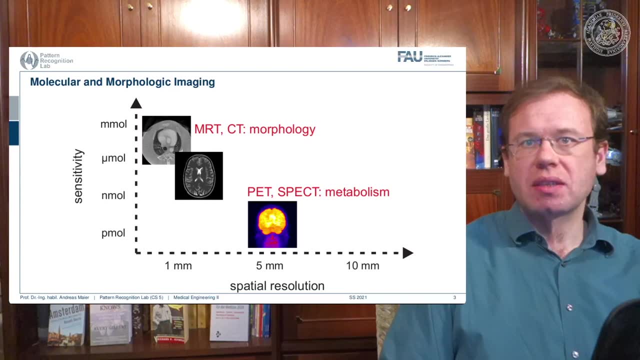 seen a lot of different imaging modalities, and we've seen a lot of different imaging modalities, many, many different modalities- and all of those modalities have very different properties. In particular, they're very different in terms of the sensitivity, so the amount of molecules or the 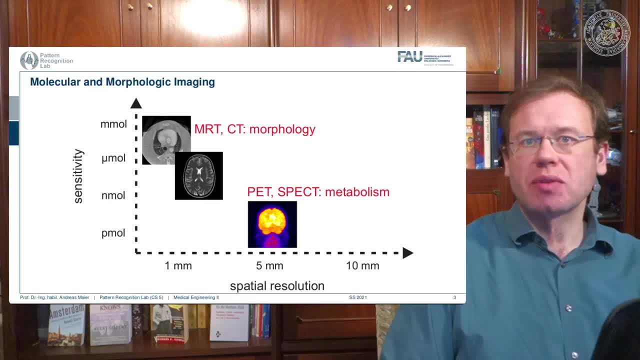 amount of different material you can visualize in terms of contrast. We've seen that MRI and CT. they need kind of lots of material in order to generate contrast, but they also have a very fine resolution. On the other hand, the, on the other hand, the nuclear imaging, like PET and SPECT. they can visualize very small quantities of tracer, for example, but they come at a coarse resolution. 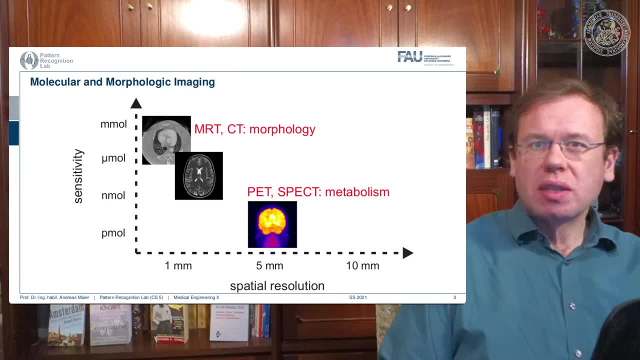 nuclear imaging like PET and SPECT. they can visualize very small quantities of tracer, for example, but they come at a coarse resolution. So you see that all these kind of things they come with certain trade-offs, and systems theory is essentially a theory that allows us to understand those trade-offs. 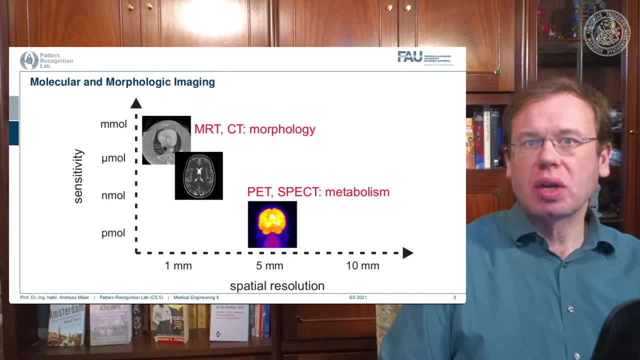 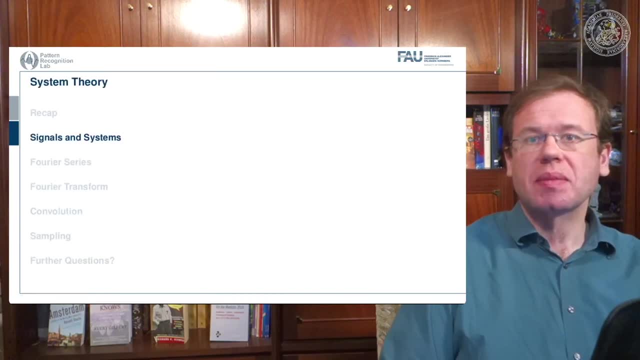 So this is generally a theory that allows us to work with different things that are processing- Let's say a Messiah, let's say information or signals. Now, if we want to understand that, we have to talk about signals and systems first. 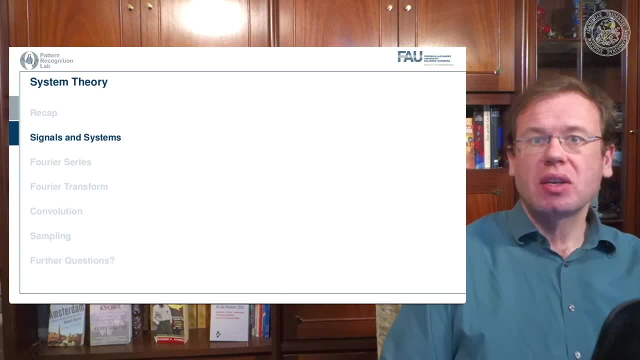 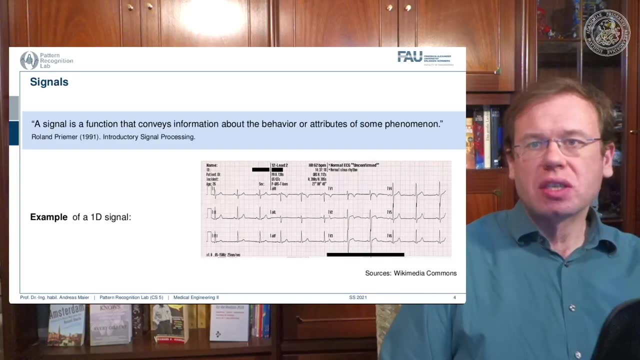 So signals and systems are the key components towards systems theory. Now, what is a signal? A signal is a function that conveys information about the behavior of attributes of some phenomenon. This sounds a rather coarse and complex definition. As an example, I brought to you here an ECG. 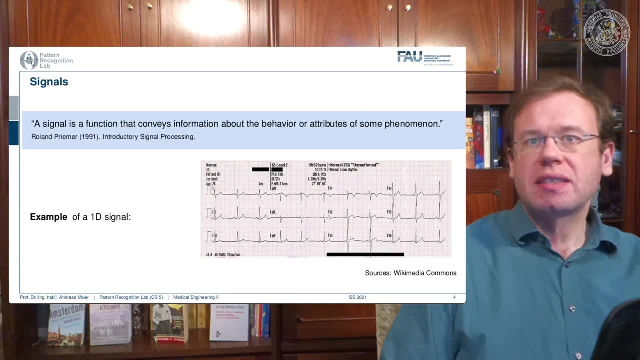 So ECG is a signal and this is essentially a voltage that is measured from the body, and we use it to measure how the heart behaves inside of your body. So this is an information. The information that we want to have is: we want to diagnose the heart and therefore, 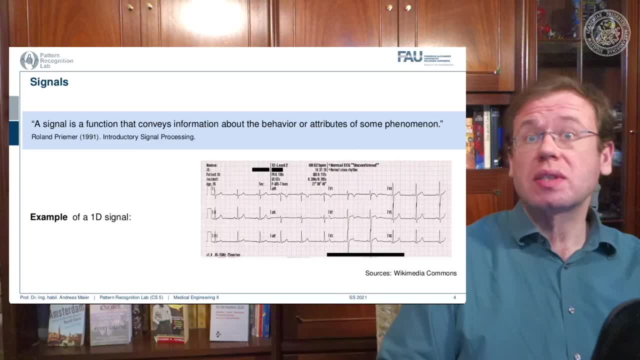 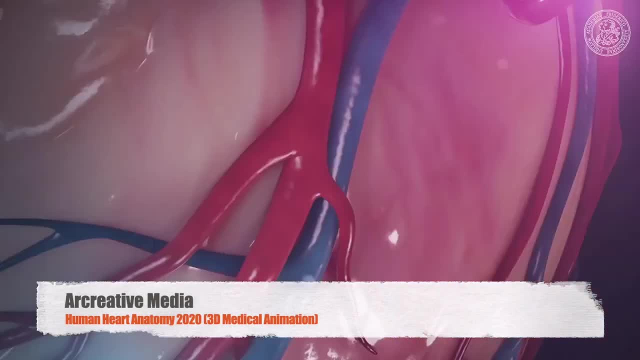 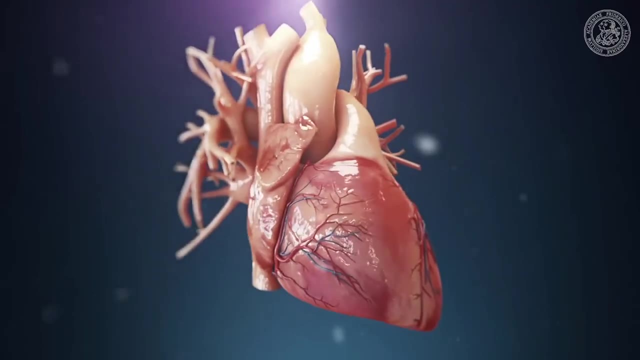 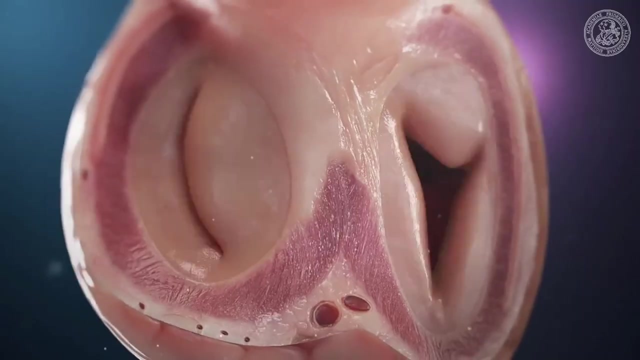 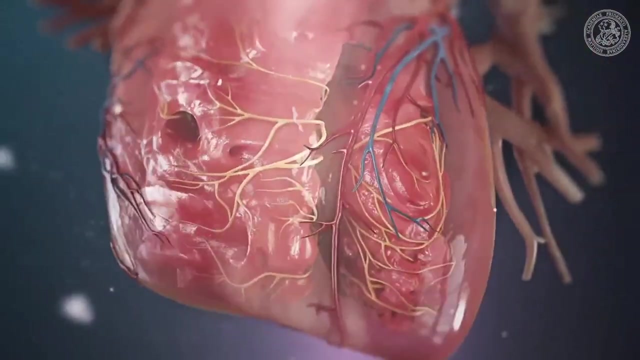 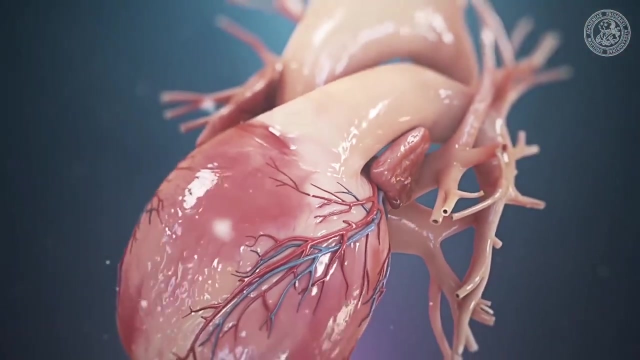 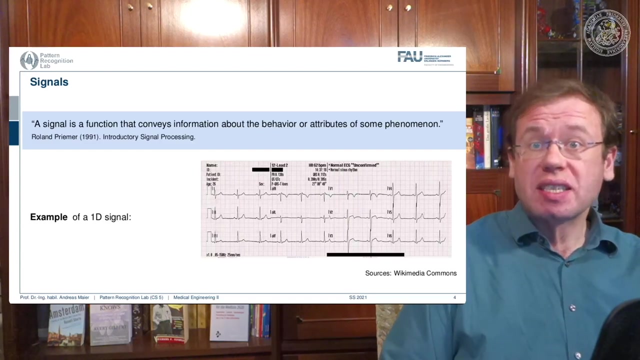 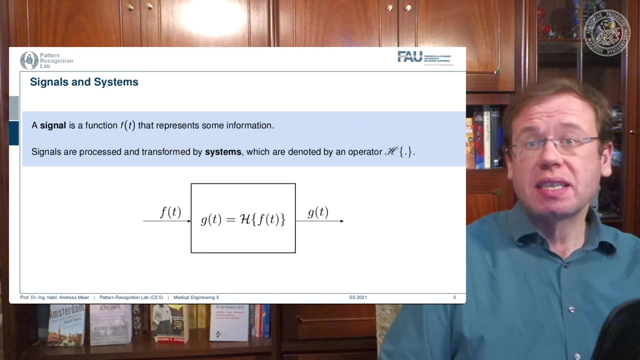 we look at the voltage that is generated by smaller signals, Small electrons that are attached to your body and they deliver this kind of signal. Now, with the system, we want to somehow process that information And, in an abstract sense, a system is something that processes the signal. 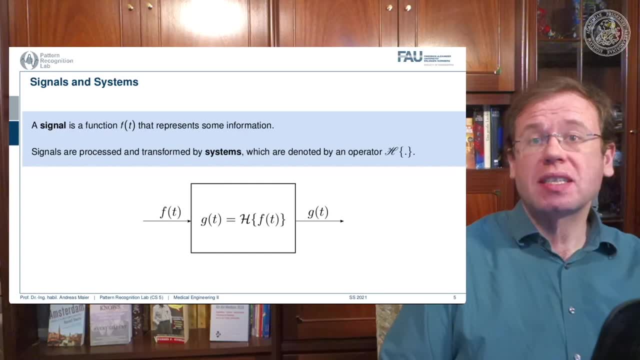 So the signal is generally a function that represents some information, And the signals are processed and transformed by systems And this is generally denoted, at least here in our lecture slides, with an operator h. So you have some function f of t. 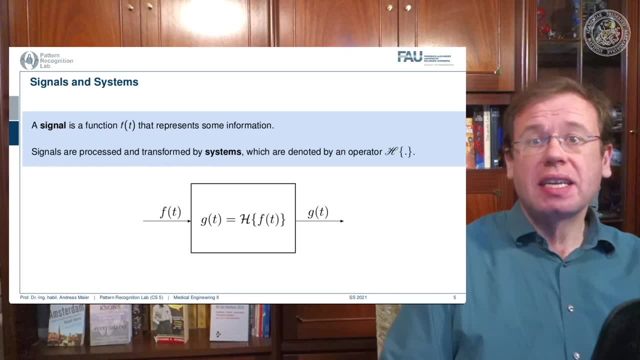 This could be the ECG that we just looked at. And then you have some system and the system processes the function, the signal, and then generates a new signal. So this is g, So we have f of t as input, We process it with our system and the system produces a new signal. 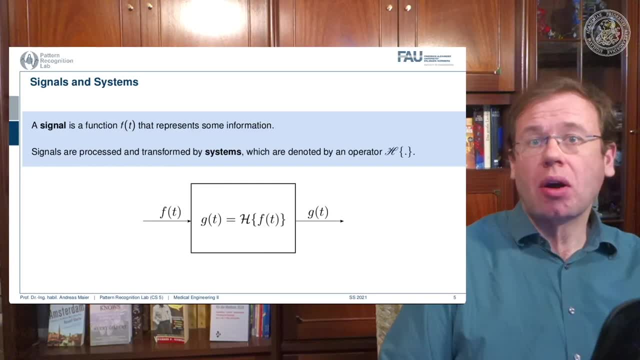 So this is the fundamental setting that we are operating in And you see that this is kind of a really big problem domain. So our system could be anything ranging from a simple sensor from the electrodes, But the system could go as far as. 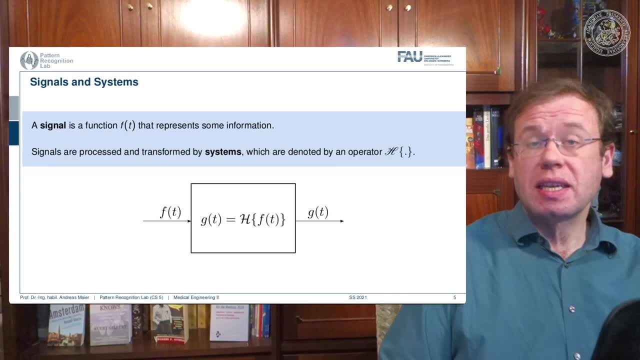 The heart that is generating the electricity that is sampled by our sensor, And the sensor is connected to a device that is then displaying the signal on the screen. So that could also be a system. So a system can be a really complex conglomerate of different processing units. 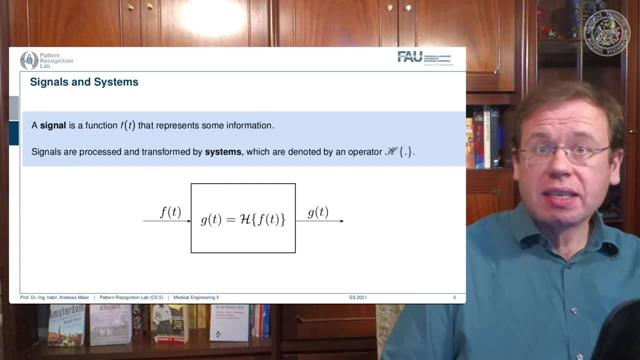 Also, if you think about modern AI techniques, deep learning and so on, they essentially also form information systems, And everything that you're learning here about signals and systems will also apply to very complex systems. Now, in order to be able to describe these systems better, we also assign a couple of 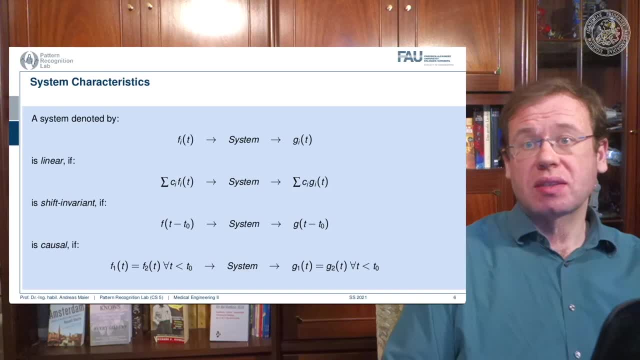 properties. So these are characteristics of systems that allow us to find classes of comparable systems, And of course we describe this with some kind of mathematics. So we can have a system, and this is denoted by our operator h. It takes in some functions, fi. 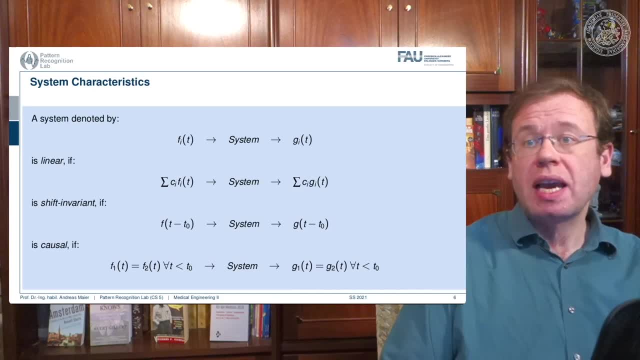 Now we have multiple functions that go in and we produce multiple functions that go out, So it's not just necessarily a single function that we're talking about, but it could also be two or three or more functions that are processed with the system. 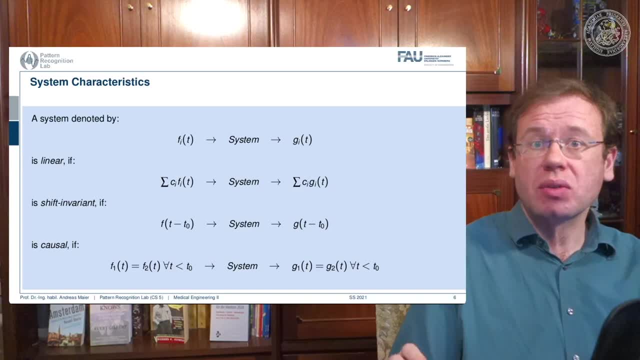 So it's. It's not just a single signal, but you can also have many, many, many signals that are processed by the system. Now, a couple of important properties are relisting here. In particular, linearity is an important one. 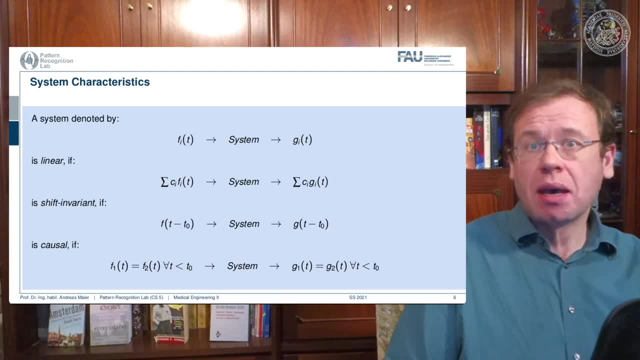 Linearity essentially tells us that if a weighted sum of input signals is processed by the system, it's again a weighted sum of output signals. So that's linearity, And we'll see. linearity is a very important property and it will help us if we are able. 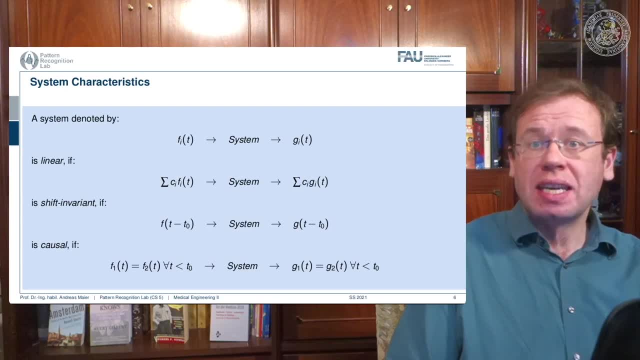 to determine whether the system is linear, because then we can also work with certain mathematics that allow us to describe the system more easily. Also, a very important characteristic is if a system is shift invariant. Now, this means that if you have a shift invariant system, 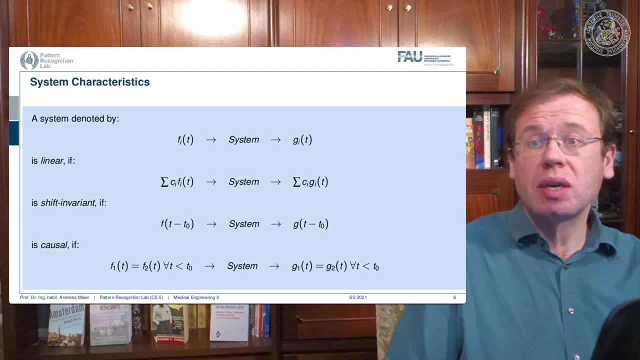 You can shift with some variable t0. And we subtract here t0 in order to shift the signal, the input signal, And if it is shift invariant, then this is nothing else than shifting also the output signal. So shift invariance means that a system processes independent of the shifting of the signal. 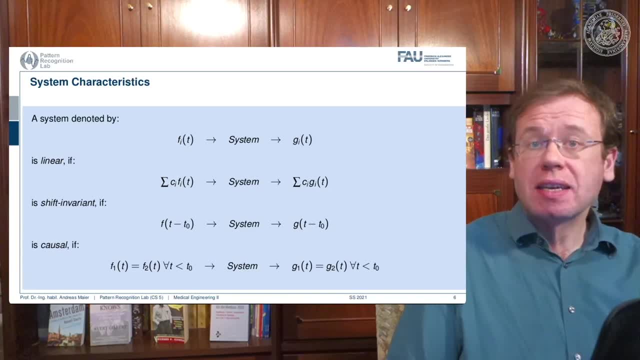 So if I shift the signal, process and get the output, It is identical to processing and then shifting. So this is shift invariance, and we'll see that linearity and shift invariance are very important properties that allow us to describe systems very elegantly. if the two properties 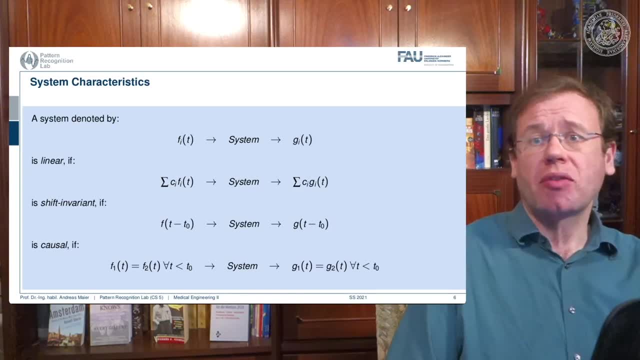 are fulfilled. We will see that in a couple of minutes, actually in one of the next videos. Another important property is causality, And here causality is A very easy concept. Causality here in this context just means that you don't have to look into the future. 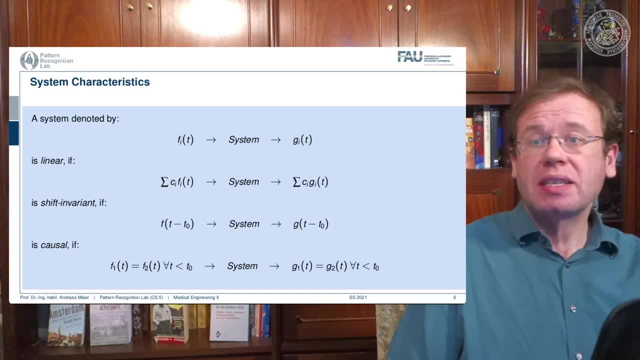 So if you have some input signal, then the system can process the input signal And it will be able to determine the output without having to access future information. So in this case the systems are causal, So we don't have to look into the future. 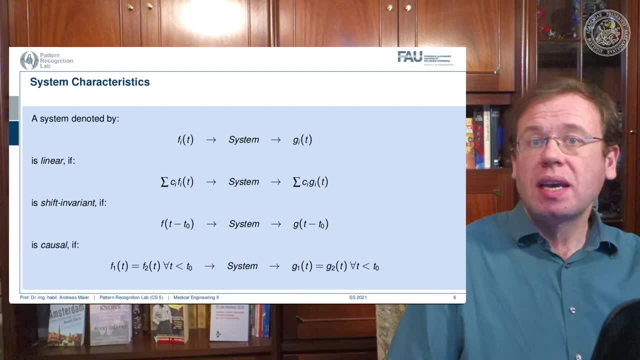 So we will Only be able to process the output and generate the output without having dependencies on observations. that we didn't do so far. So you can imagine that this is a very important factor if you think about latency and dependency of systems on future observations. 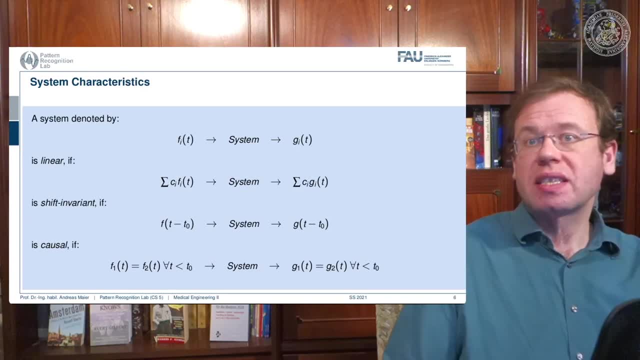 If you would have to look ahead, then this can cause a significant delay in the output of the processing system. If you have image processing, Then Causality is not such a big issue, because you typically have access to the whole image domain and then it's only a 2D shift and we can do that in arbitrary directions. 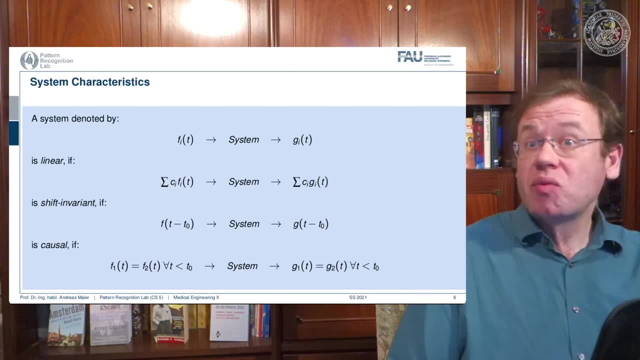 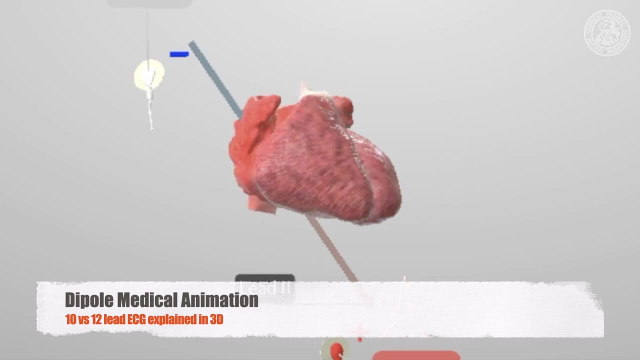 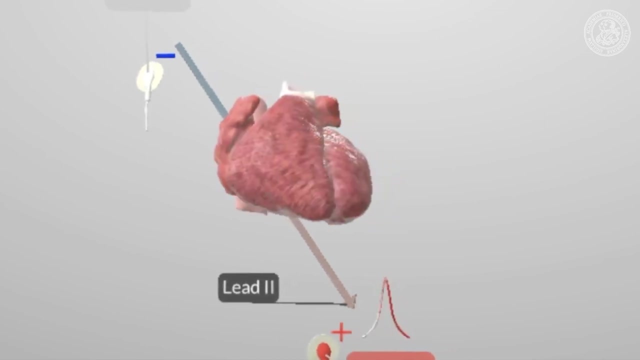 So there, causality is not such a big deal. It would be if you have moving images like videos, then causality is again a huge issue. So you don't want to be dependent on future time points. So let's take a look at some of the things that we can do in the future. 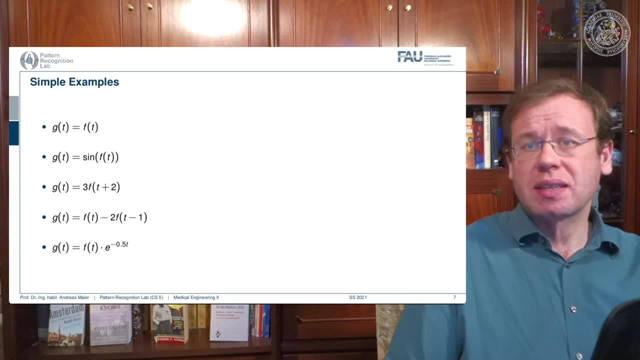 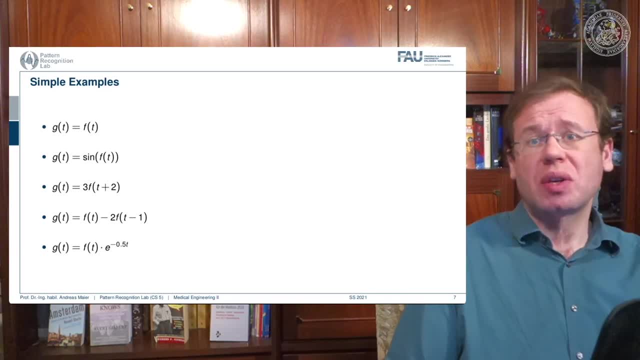 So let's look at some of the things that we can do in the future, And I have here a couple of examples. The first one is very easy. So the output of the system GT is simply the input of the system. Then a second one is that we have the sign of the input function. 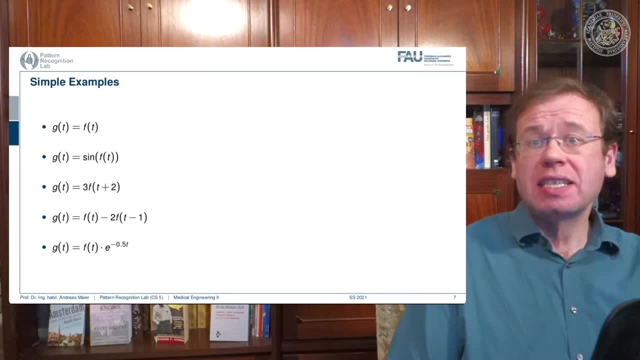 The third one is that we shift by two and then multiply by three, So that's also rather easy system. The fourth system is that we essentially duplicate the function, So we have the original function minus two times the function shifted by one. And the last one is we are multiplying with an exponential function that is dependent. 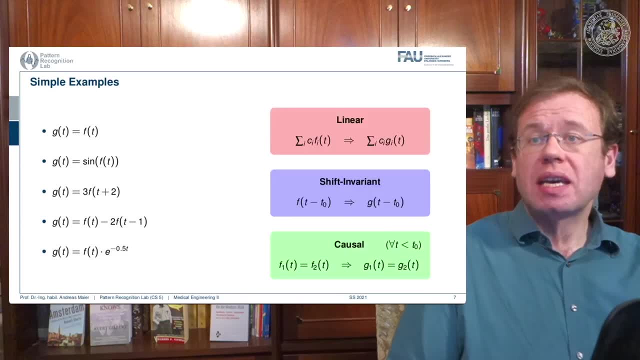 on t. So let's look at those examples and see if we can apply here our different properties and see whether they apply. So the identity is a very simple case and we can see if we have the identity. essentially, the linearity already falls out of this. 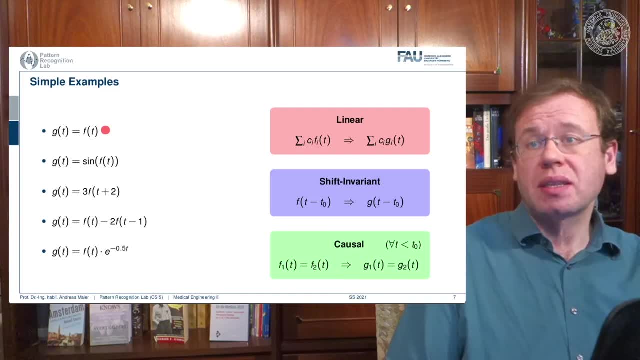 So we could just plug this in and prove linearity. No big deal. This applies. Shift invariance again also applies. So if I shift before and after, it wouldn't do anything, because we are just using identity here. So this is a linear and shift invariant system. 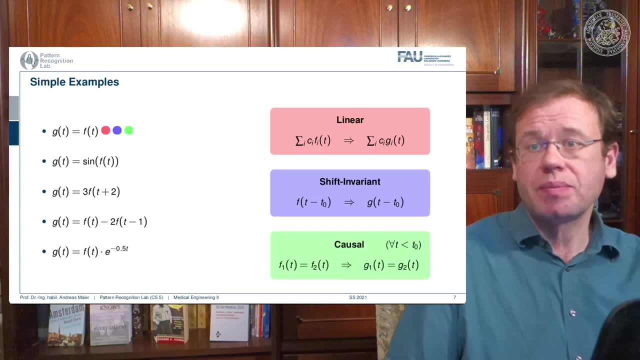 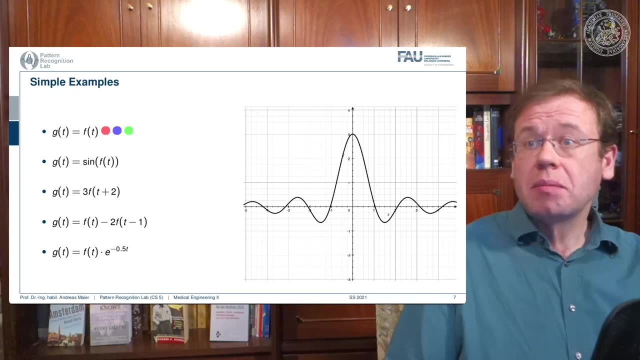 And of course, it's also causal, because we don't have to look into the future. Let's still look at an example, And the example that I have here It's not the easy one, It's the ECG, because I'm using a function plotter here and you know the ECG. I would 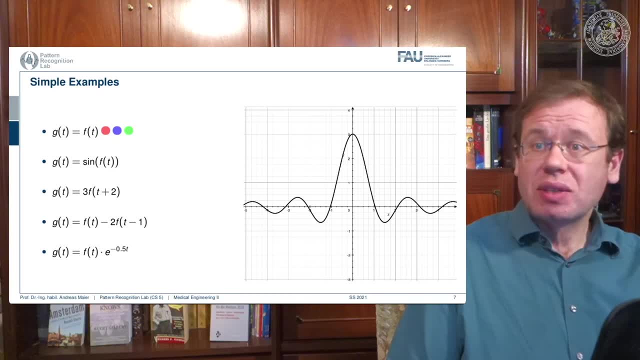 have to plot from data and therefore it's easier to take a different function. Here I'm using a sinc, So this is nothing else than a sine of x over x, And you see that this is then essentially a sine that is also amplified here by the. 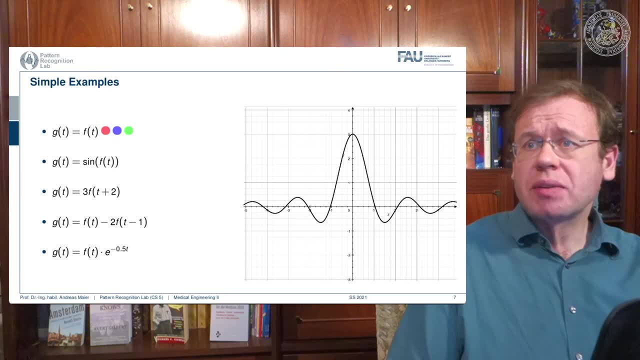 way with a factor of three. But this function- here We can see that it alternates. It alternates up and down and it also dampens, because we're dividing by the magnitude of x towards the outside. So we kind of can very easily see whether it's shifted or not. 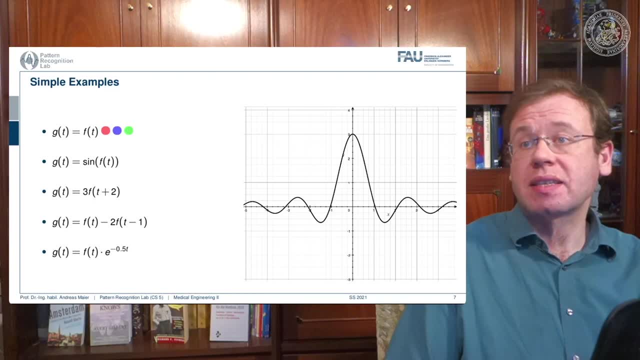 So that's very nice about this function and this is why I'm taking it as an example, as input for the other systems that we'll see in the following. So, of course, our identity does nothing. if I shift, You can actually see that I'm plotting. 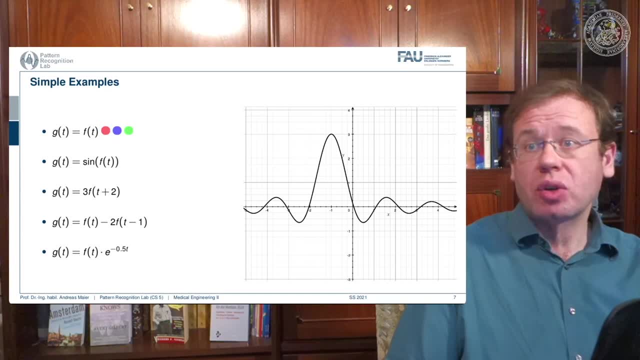 I'm plotting two functions here. I'm plotting a dashed version and a gray version of the same function and you see both of them of course overlap because we have identity. and obviously, if I shift this a bit to the front and back, you see both of them still overlap, of course, because of the shift invariance. 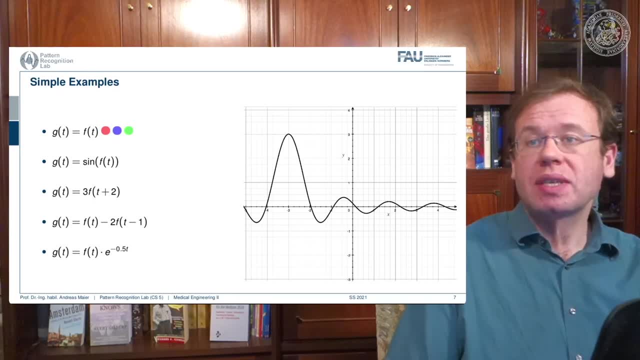 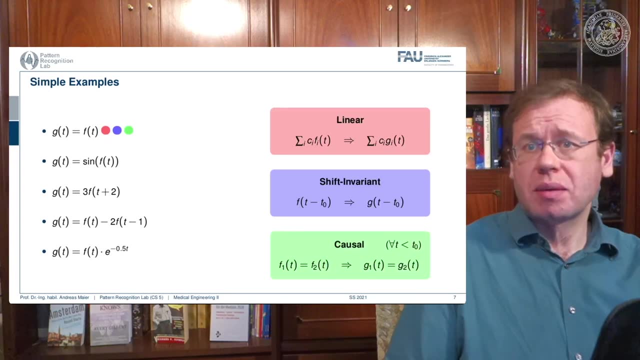 So no big deal. All of the properties apply and we can see this in this nice visualization here. Let's make this a little bit more complicated and go to the second example. We have the sine of the input function, and this is a bit different. 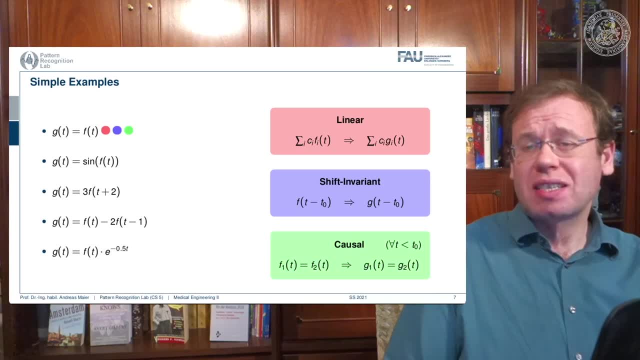 So if you think about the linearity, the sine function has a maximum value of plus one and a minimum function value of minus one. So whatever I'm doing to this kind of function, I will be clamping to minus one or to one. So this is not a linear function. 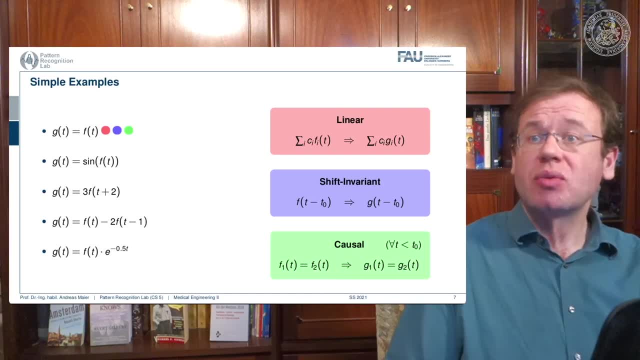 Because if I have a superposition Before applying the sine, the result will be different than applying the same superposition or weighted sum after the sine. So this is going to be different. Linearity does not apply. How about shift invariance? 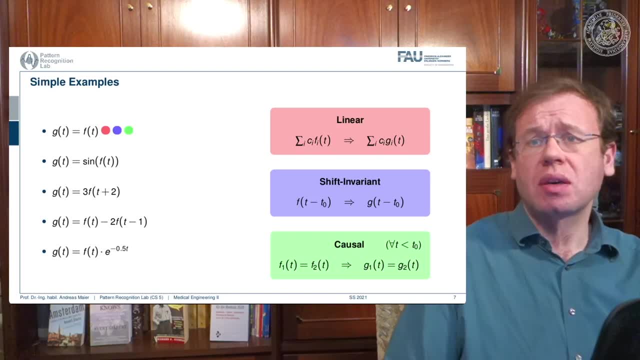 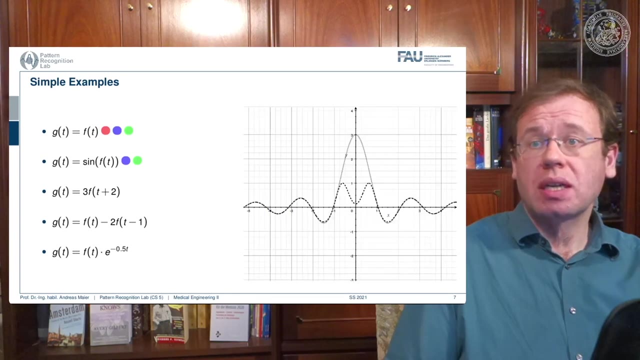 If I shift the sine, well, the function is shifted. So shift invariance actually holds. So our function will be shift invariant. Also causality- I don't have to access the future here- So also causality will hold. Let's look again into the example. and I brought again our sinc function. 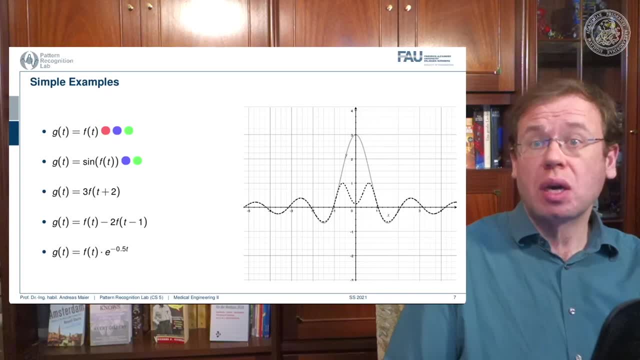 Now you can see that we have two different outputs. So the output, our g of t is dashed, while we have in gray the input function. And you can see here that exactly this clamping effect is taking place. So the values that are above one, they get essentially transformed and they are mapped. 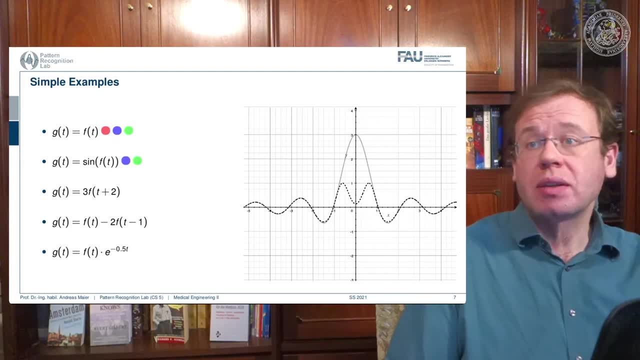 into a different space, so that we essentially get rid of the central lobe here by applying the additional sine. Now, how about the shift invariance? Let's shift the input and if you see I'm shifting the input, I can shift it a bit around and it doesn't change anything because it's shift invariant. 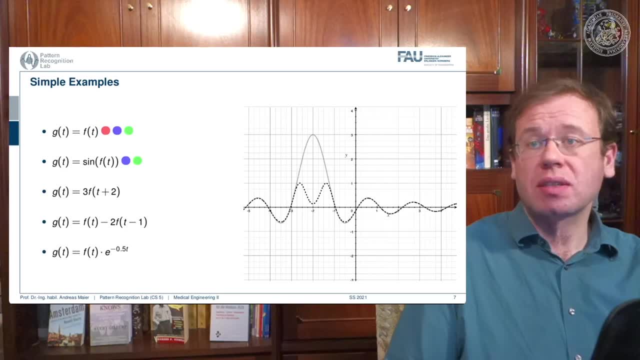 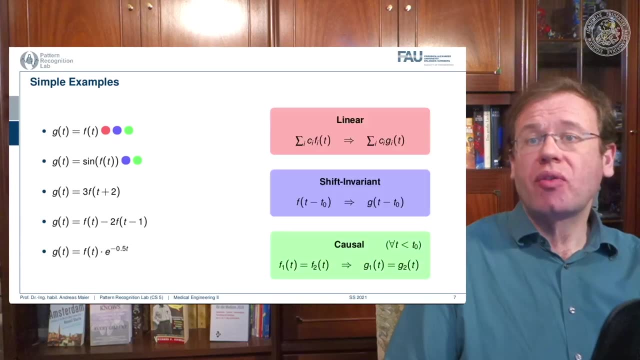 So we don't have a problem here, and it's also causal, because we don't have to access the future. Well, let's go to the third example Now. the third example is just multiplying with three, and then you have a shift of plus two. 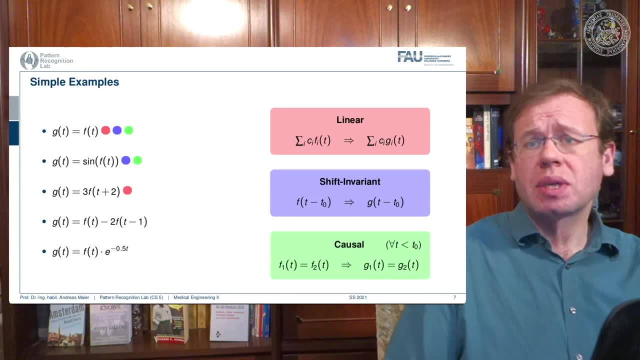 So this is actually linear, because we just have additions and multiplications, Not a big thing. So our superposition or weighted sum would not be changed. That's good Then this is also shift invariant, because I can shift before and after. it doesn't change. 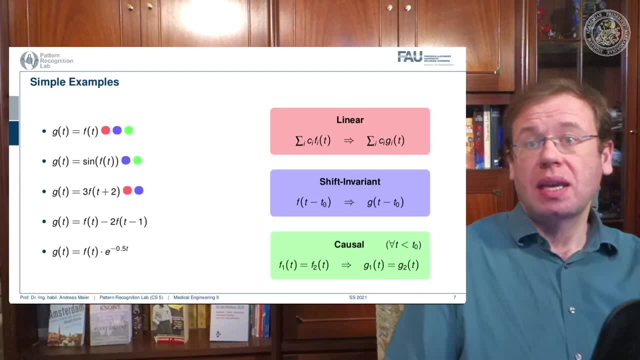 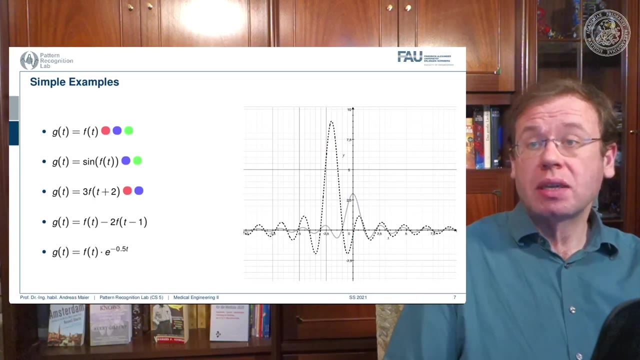 anything but it's not causal. I add two in the index, which essentially means that I have to shift the function into the future. So this is a non-causal example And you will see that here on the next slide. You see that our central lobe of the sink is moved to the left. 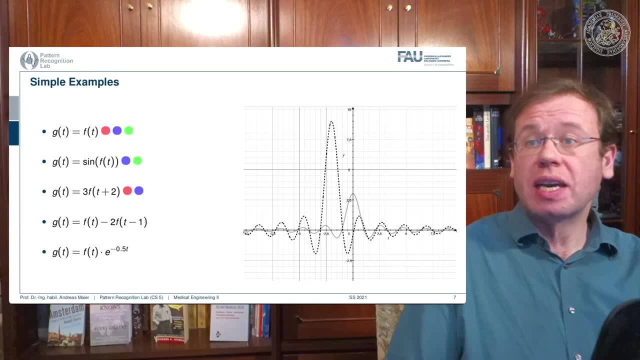 So if you compute the output of the system, you have to access the future. So this is a non-causal system. Again, it's shift invariant. So if I shift the input, also the output will be shifted. So that's not a big deal. 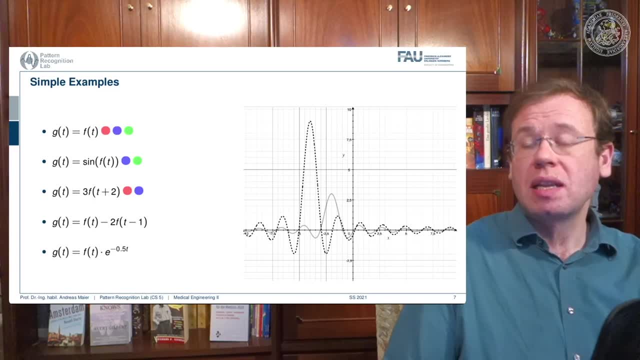 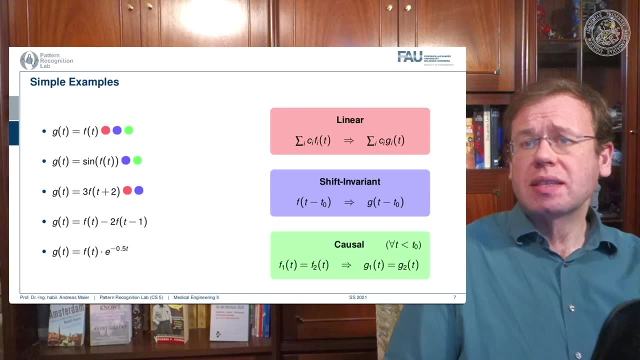 So here we have an example for something that is non-causal, linear and shift invariant. Let's look into the next example. So the next example is again: we subtract two functions from each other, so it's actually the same function We shift, we multiply by two. 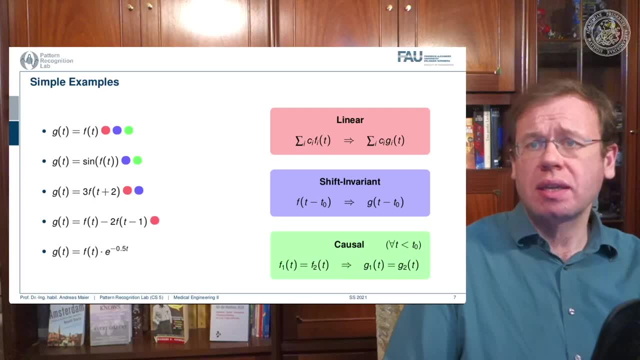 No big non-linearities in here, so this is actually a linear system. You also see that it is shift invariant because we don't have any functions in there that cause any problem with shifting, And you will also see that it's causal because we don't have to look into the future. 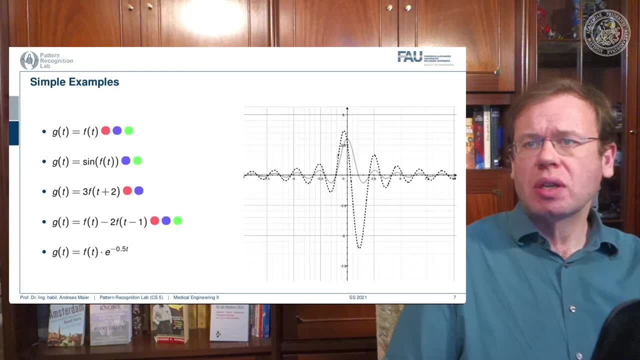 It's a slightly more complex system. If you look now at the plot, you can see our input is again the sink and our system now shifts by one and then subtracts two times the function value, which causes this strong negative peak on the right hand side here. 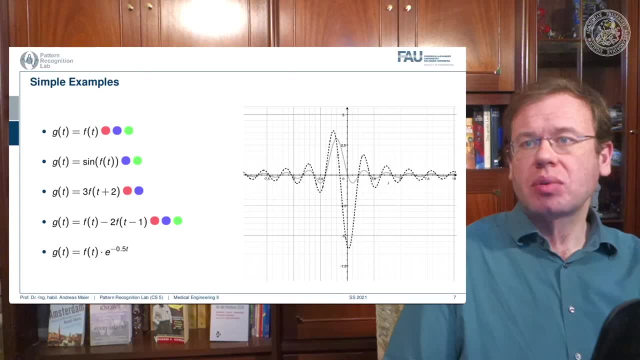 Still, it is shift invariant, So if I shift the input, the output will be shifted as well. So that's not a big deal. And we found again a system that looks slightly complex so we can express in terms of shift invariant, linear and causal systems, quite a few complex systems. 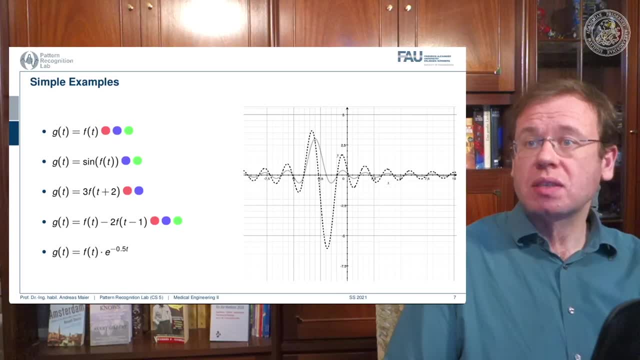 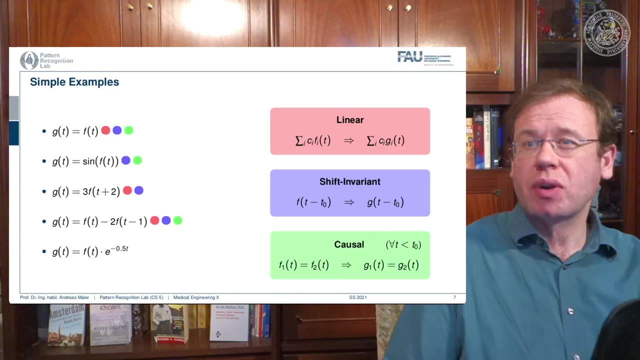 But we are still able to assign these properties. so this means that we are holding all of the three properties that we have learned so far. Now let's go to the last example, And here we have this exponential function that is multiplied, And if you remember how the exponential function looks like, you see here with the negative. 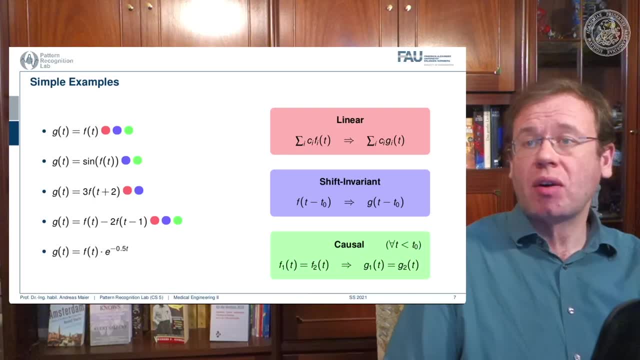 exponent. this is essentially a decay. So everything on the right half space of our coordinate system, everything here, will be dampened. On the other hand, everything on the left hand side will be amplified And the t is not dependent on the actual shift. So this is neither linear, because we have the exponential function. 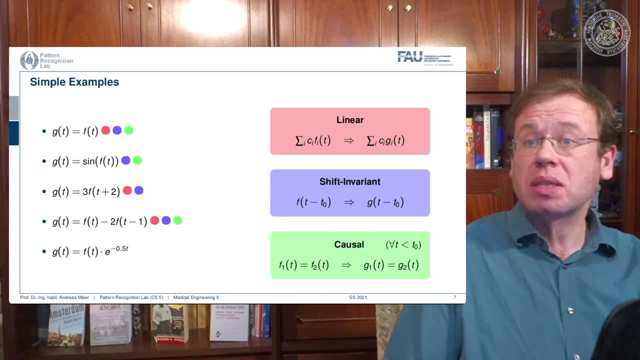 And the exponential function is dependent on t but not on the shift of the function, So it will also be shift invariant. So it's also not shift invariant, but it's causal. So this is the only thing that applies to this system here. So let's have a look here. 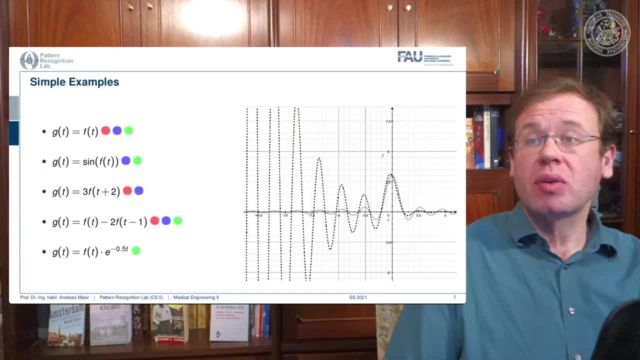 And, as I already said, you see the dampening on the right hand side of the half space and you see the magnification, The amplification on the left hand side. So, although our sink is essentially just leveling out, you see how the exponential function is. 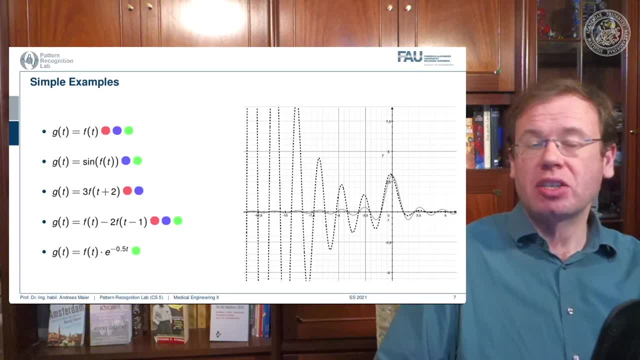 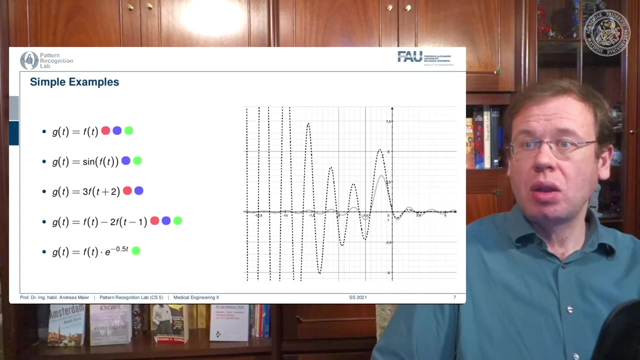 boosting this up. So this is really an amplification that is happening on the left half space. Now the key problem here is that the amplification is fixed to the coordinate system and not the function. So if you look now at the shifting, you see that our lobe gets amplified more and more. 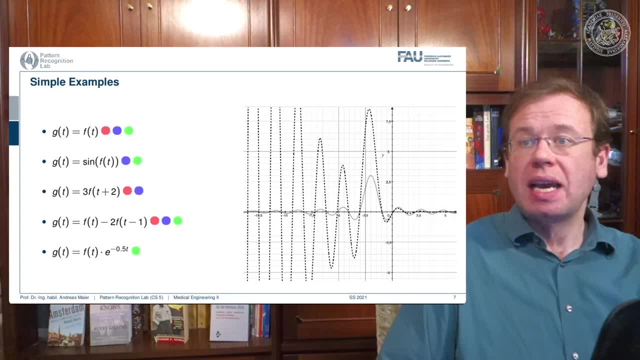 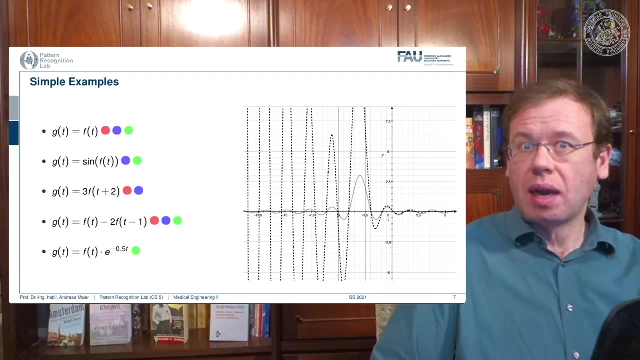 And further we go away from the zero position, And this is very interesting. and here you see a system that is definitely not shift invariant, So it processes the data very differently depending on how you shifted it. So you see how shift invariance is also a very important property if you want to describe. 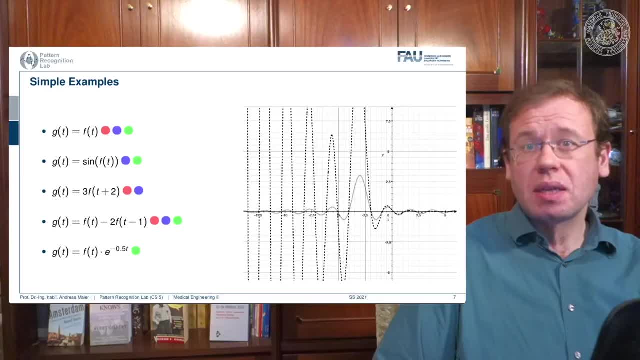 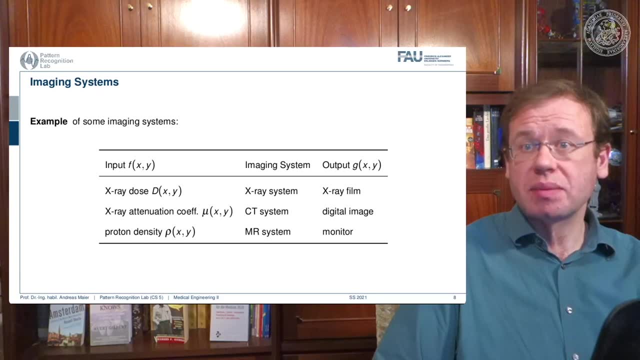 systems Fascinating. Now let's summarize a little bit what we've seen here so far. So we've seen that we have different systems. They can be anything from analog processing to digital, So it could be x-ray dose entering your detector. 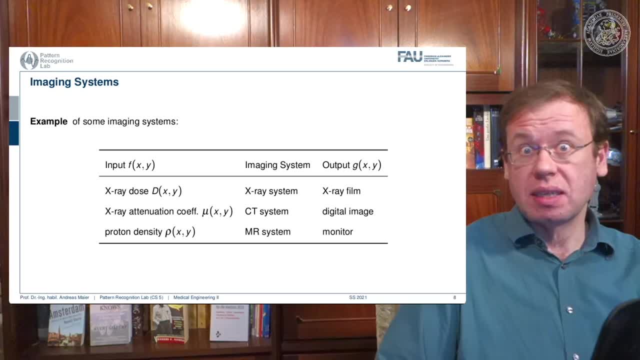 Then the x-ray system and then x-ray film. So all of this is analog. It's still a system. System theory applies. It could also be attenuation coefficients, and then you have a computer tomography system that is, computing digitally The entire image. 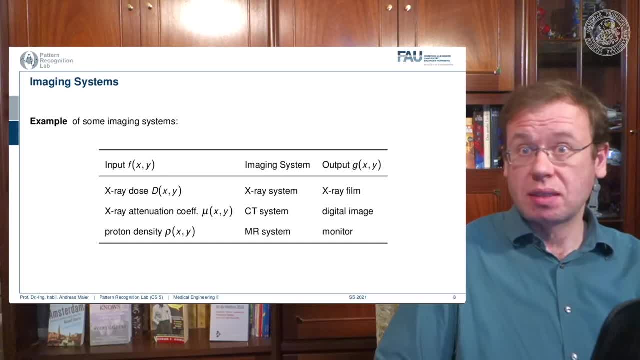 And then you have a digital image. It's also a system, System theory applies And it could also be something like proton density, an MR system with all the RF coils and so on. Really complex system And still it would be modeled by our system theory. 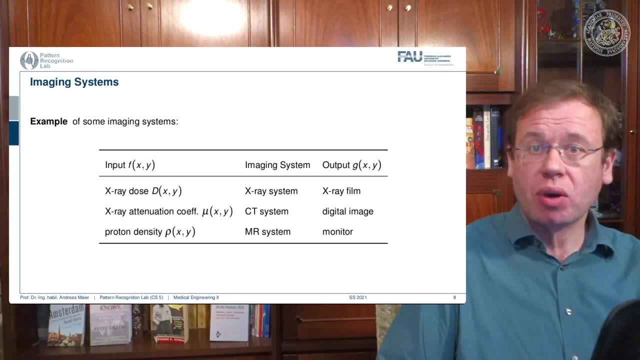 So you see why system theory is very important for our field And, to be honest, You will need this throughout your entire career. System theory will apply, So this is truly fundamental to anything that you want to do in medical imaging processing systems, So please take care. 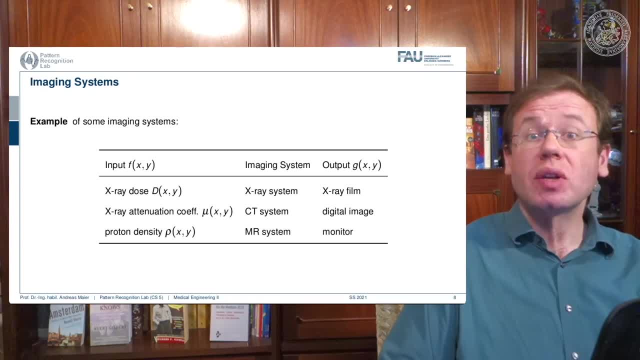 The next couple of videos will be very important And you will hear this over and over again in your studies. There will be several people trying to explain this to you And I hope this rather superficial way is a good start, And I hope you dig into all of the math in order to follow the systems theory. 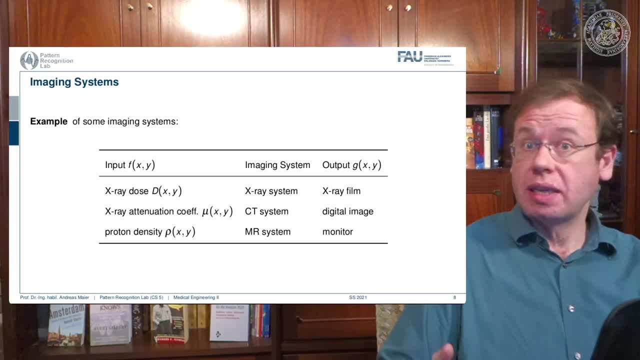 By the way, also the complex AI systems and so on, they also obey systems theory. So it's not like that you can trash it if you use deep learning or artificial intelligence and so on- All the systems that are built on such techniques. they also have to obey systems theory. 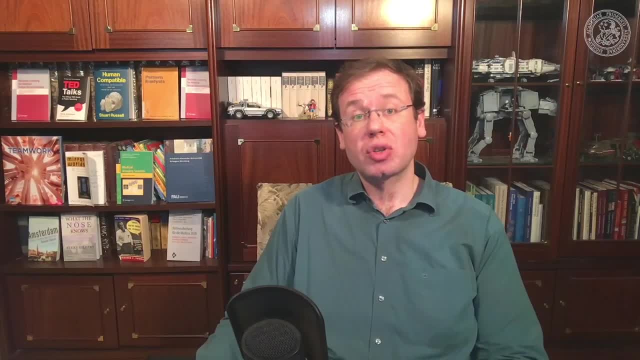 Well, I hope you liked this short video and an introduction. It's very short, it's quite superficial. You've seen a little bit of the math. We introduced two very important concepts, no, three very important concepts, That is, linearity, shift, invariance and causality.